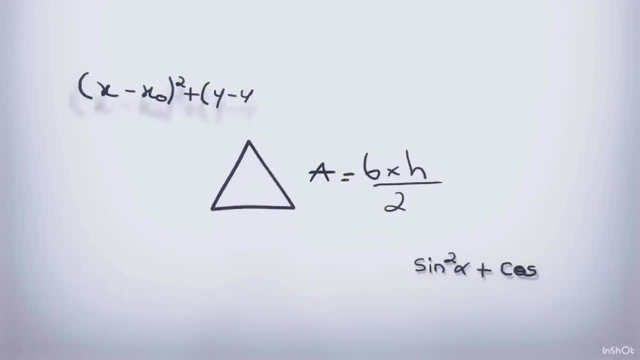 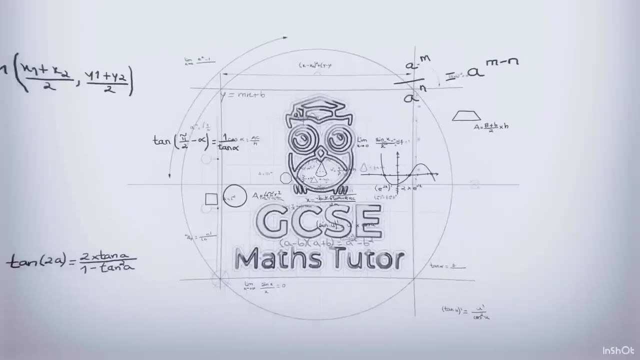 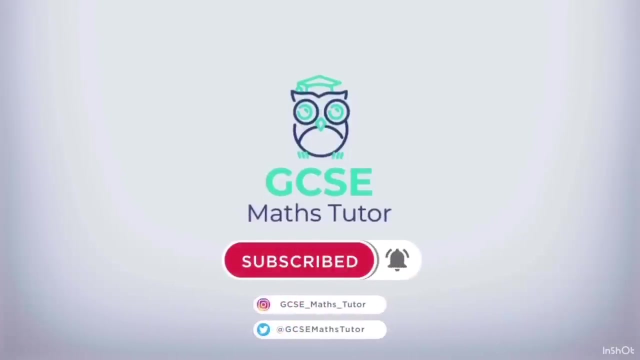 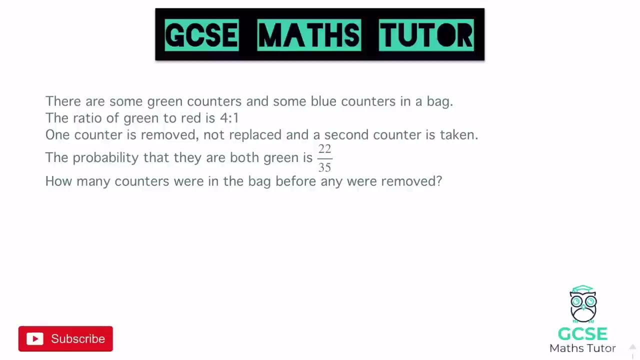 Right, okay. so in today's video we're going to have a look at some probability equations. This is quite a tough topic, okay, and the way I'm going to structure this video is I'm going to do one question, then you're going to do a question that's fairly similar, So do grab a piece of. 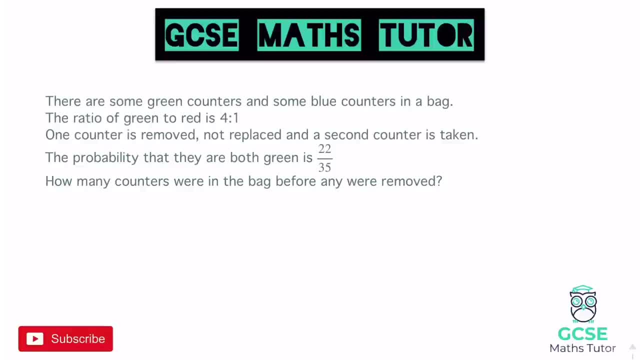 paper. grab a pen, make sure you make some notes on these questions that I go over, because you are going to have a go at one and there is some quite extensive mathematics going on in these types of questions. okay, You're going to have to have a very good understanding of probability. 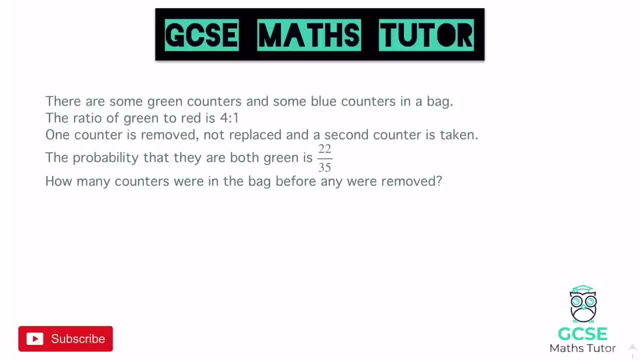 trees. you're going to have to have a good understanding of creating expressions in algebra and forming quadratics, solving quadratics, okay. so there's a lot of maths going on here. I'm going to link as many of those topics as I can in the description, so do make sure you check those out. 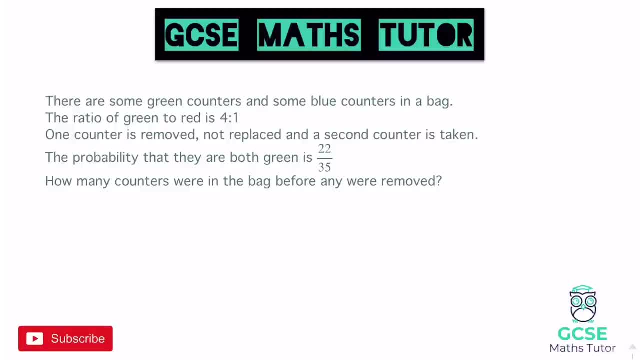 if you're not sure on any of these, But we're going to get started, Okay. so we're going to have a look at this question here. and it says there are some green counters and some blue counters in a bag and it says the ratio of green to red is four to one. 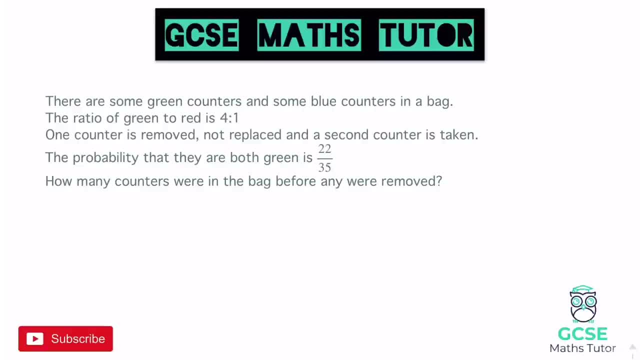 One counter is removed, not replaced, and a second counter is taken, and that's quite key there, that it's not replaced And it says the probability that they're both green is 22 over 35.. How many counters were in the bag before any were removed? So if we start to construct a probability tree, 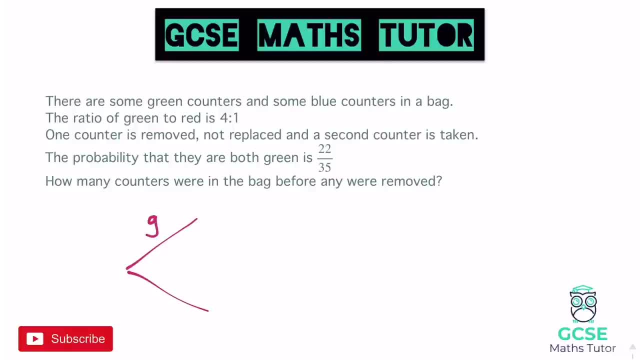 here and we have a look at the probability of green and blue. Now we only know the ratio there. we don't actually know how many are in there. so if we have a look at this as a ratio, we've got green to blue and it's four to one. We don't know how many lots of four and how many lots of one. 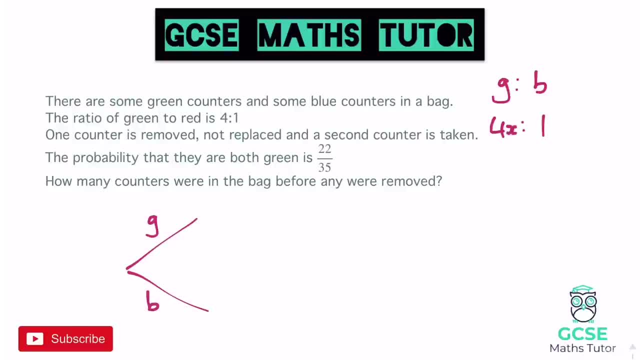 so we can allocate some algebra to this. We can say: it's four x four lots of a number, and one lot of a number, one x. So if I were to actually start writing this as a probability, I first need to know what my denominator's going to be. So add these both together. 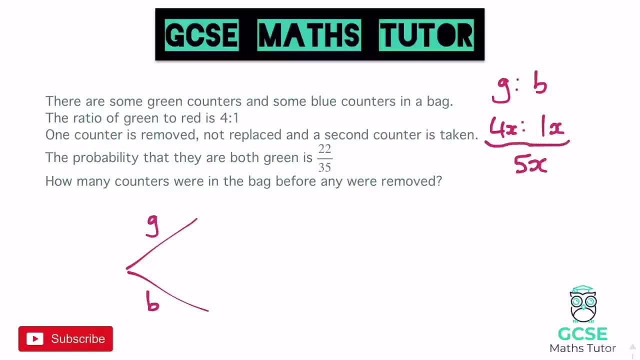 and we have five lots of x as our total amount of counters there. Now we can construct these two fractions. So green is the four x out of a total of five x and blue is going to be the one x. Let's remove the one there. 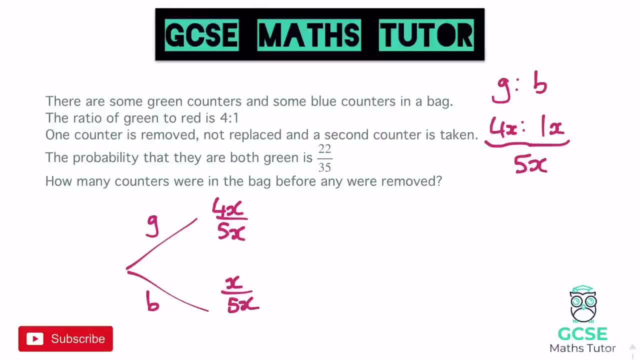 And that is again out of five x. We actually don't need to construct the full part of the tree here, because what we're actually interested in is the probability of them both being green, So really only need to look at the up part of the tree for this option. here where it's going to be. 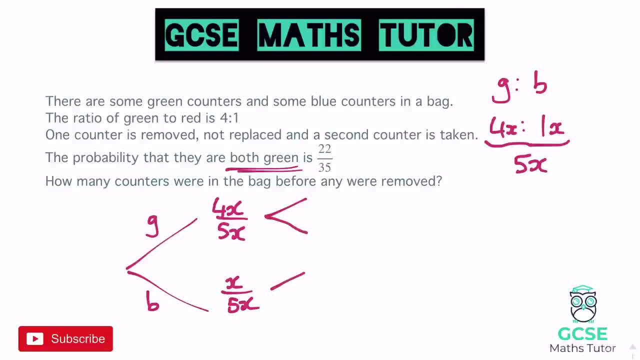 green, green, but I'm going to go about constructing all the tree to start with anyway. Okay, I do think it's important that you're able to construct these and create these expressions, so I'm going to label this up green and blue and we'll just think about what all these probabilities are. 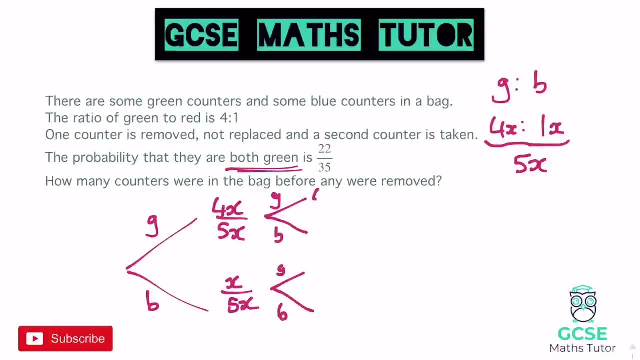 going to be Now. if I take away one of the greens, I've got four x and I'm going to take away one of them. So I'm going to get four x minus one, and on the bottom I'm going to have five x again. 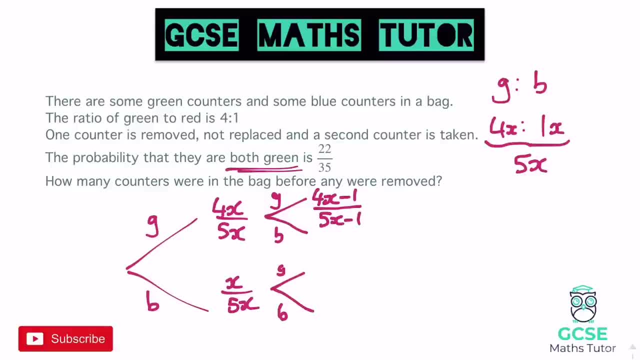 taking away one counter because one of them has not been replaced Now. they're the two that we're actually interested in, but we could go about constructing the ones below, So blue would be the one x again over five x minus one. I'm moving down here, so let's write that in. I'm going to. 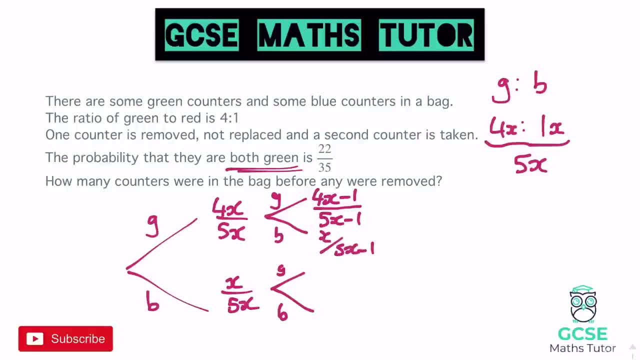 get rid of this in a sec, but it'll be x over five x minus one again. If we took a blue out, the blue would go down to x minus one and that would be over five x minus one. Green above that would stay the same, so it'd be four x and it'd be over five x minus one. 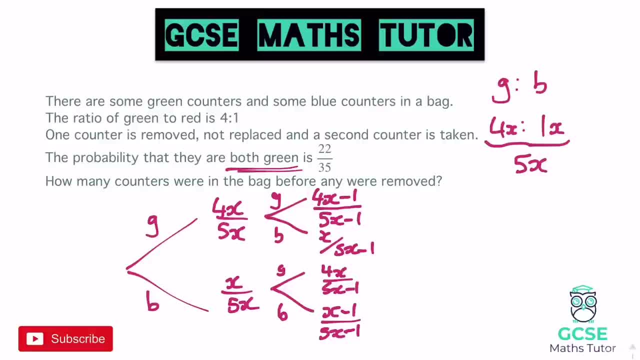 So I mean that's all the potential branches that we could have. but again, we are only actually considering the green green option here because we've been given the probability of green green. So if I went up the green and up another green here, we would go through those two fractions. 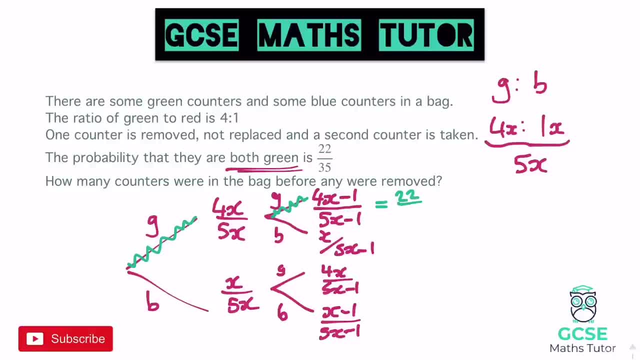 and they would equal 22 over 35.. Okay, now, what I'm going to do is I'm just going to get rid of the rest of the tree, because that's all we're really concerned about. You can save your self a lot of time here just by constructing part of it, but it's good to be able to construct the. 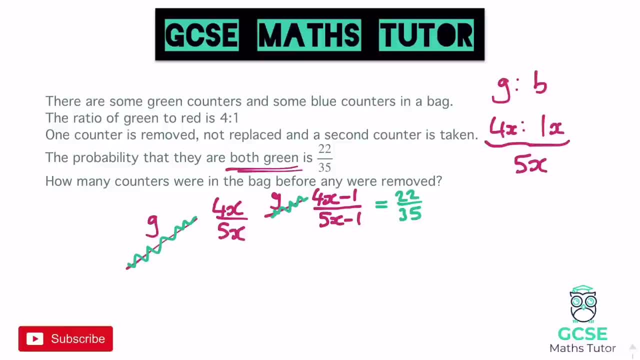 entire tree there and think about what you'd actually get Now if we do get rid of all of that. obviously, when we're going across a tree, we multiply, so we need to multiply these two fractions together. So we have four x over five x, and that is going to multiply by four x minus one. 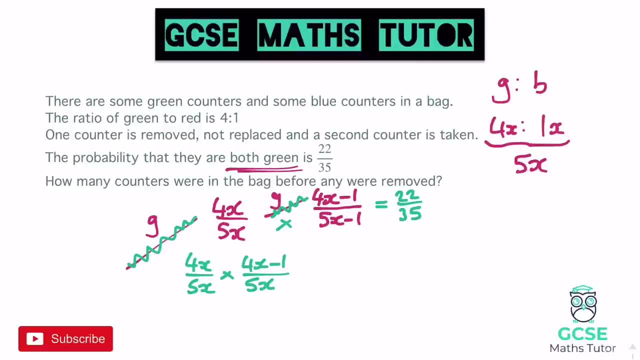 over five x minus one. There we go, and again that is going to equal 22 over 35, but before I set it equal to 22 over 35, I'm just going to work this out. On the top, we have four x multiplied by the four x minus one. Four x times four x is 16 x squared. 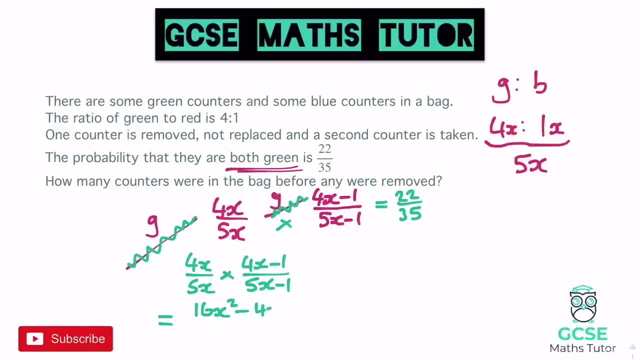 and four x times negative. one is negative: four x. Okay, just multiplying the top there, just like a single bracket, And on the bottom we've got five x times the five x, which is 25 x squared, and five x times the negative one, which is negative: five x. And now that equals 22 over. 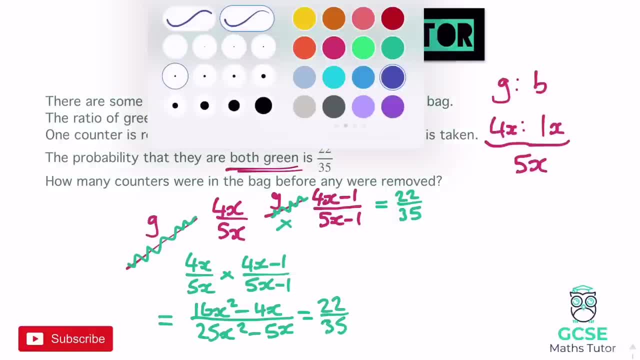 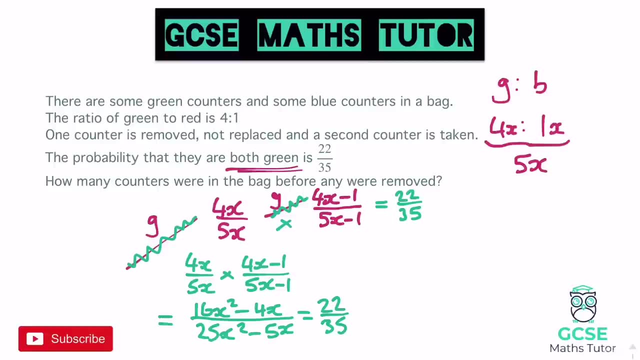 35.. So what we've got? we've got a fraction on both sides of our equation and in order to remove the denominators from both sides, we're going to cross, multiply. So I'm going to times both sides by 35,, which is going to move. 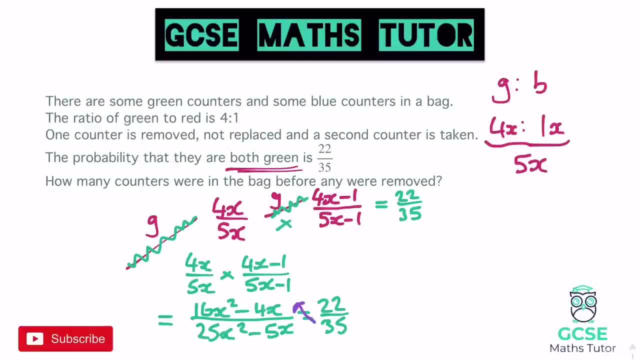 35 up to the top. here I'm going to times both sides by this: 25 x squared minus five x, which is going to move that up to the numerator over here, And if I write that all out in one step, we have: 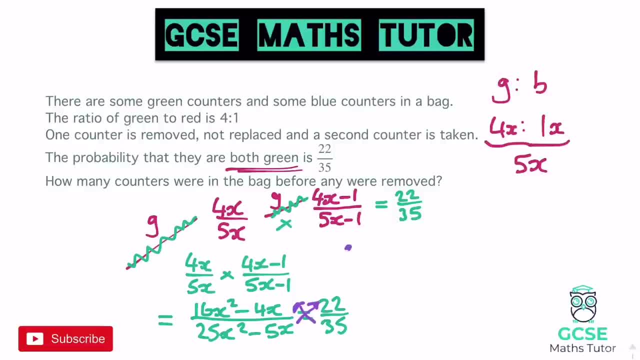 35 lots of the left numerator. So we have 35 lots of 16 x squared minus four x. that now equals 22 lots of the 25 x squared minus the five x. Okay, so I've just cross multiplied there, just so I've got a single line equation. Now what I want to do is actually just remove. 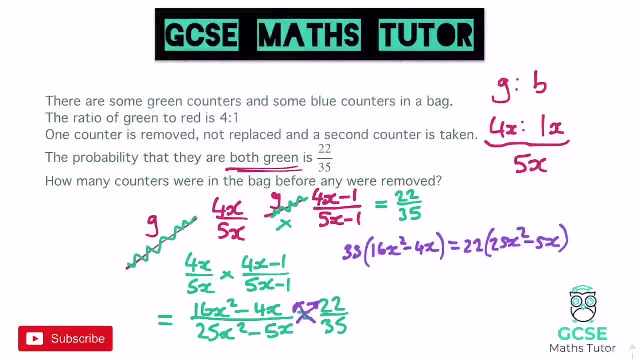 these brackets. So I've got some quite big numbers in here. The one you're going to do is not so big, but if I actually multiply these brackets out 35 times 16 gives me 560 x. squared minus four, lots of 35, which is 140.. So minus 140 x, Oh, there we go: 140 x And that equals 22 times. 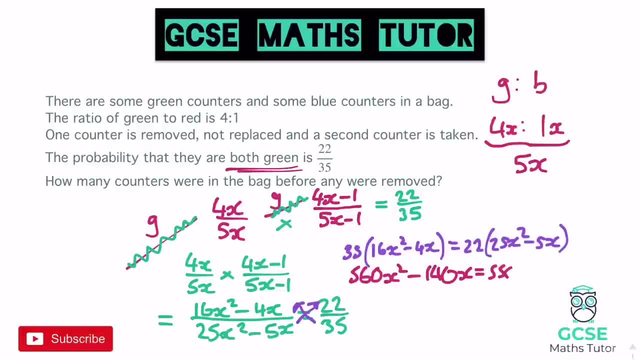 25,, which is 550 x squared minus 22 times five, which is 110 x. There we go. Now we can actually rearrange this so we can get everything on one side. So we've set it equal to zero. So if I 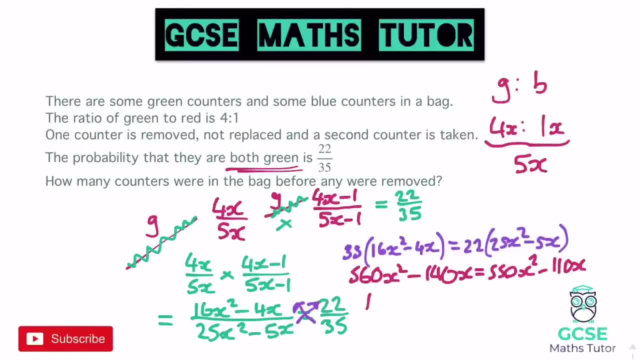 subtract 550 x squared, that's going to be 560 x squared. So that's going to be 560 x squared From both sides. I end up with 10 x squared over here. And if I add 110 x to both sides to get rid, 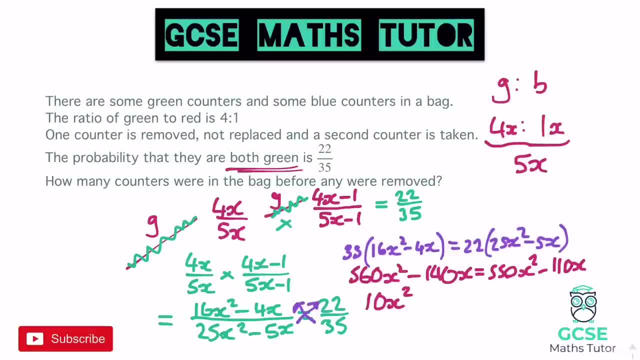 of that, negative 110 on the right, if I add it to negative 140, I get negative 30 x and that equals zero. Okay, now it equals zero. We're just solving a quadratic here, So there's a couple of ways you. 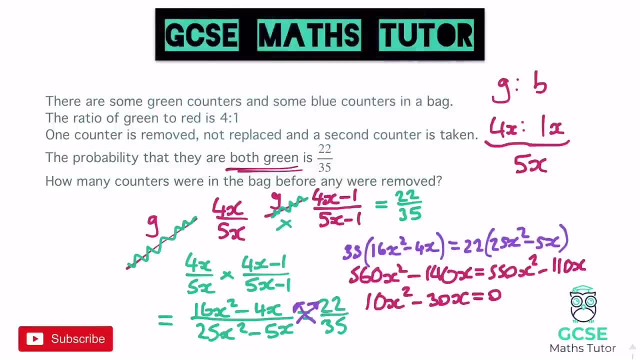 can go about it. You can solve it as it is or we can simplify it. first I'm going to divide both sides by 10.. So if I divide everything by 10, we get x squared minus three. x equals zero, And I'm going to just remove some of this working out here. So hopefully you've. 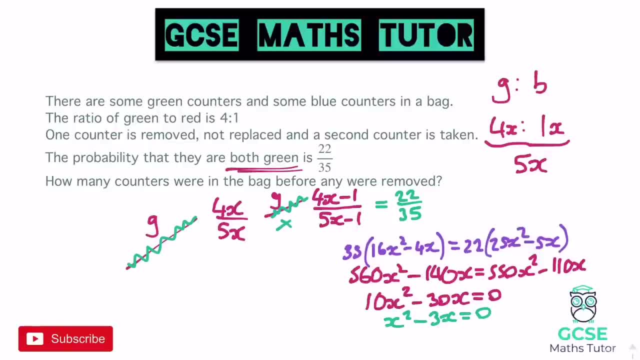 written this down. I'm going to remove this, get rid of this and just bring that up here. So at the moment we have x squared minus three, x equaling zero. Now, whenever we're solving a quadratic here, we need to factorise it. This doesn't factorise into a double bracket, but we 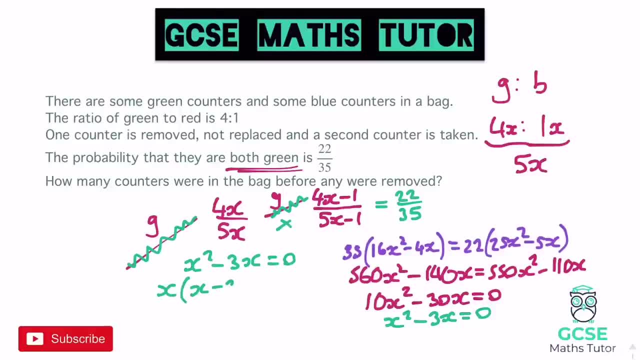 can factorise x out. So we have x brackets. x minus three equals zero. And we have our two solutions here. We've got the one in the bracket, which is x equaling positive three, not neither negative three, And on the outside here we've got x equaling zero. So we've got two answers. We've 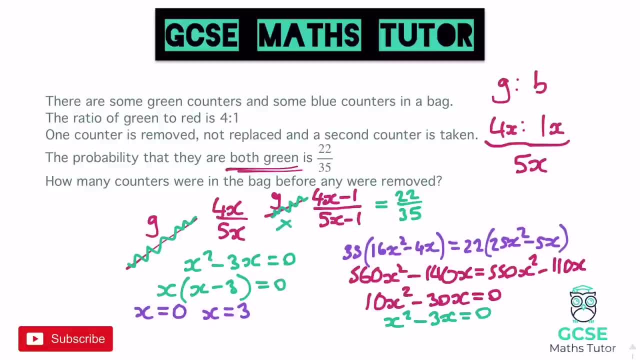 got to decide which one. it is Now x in our case. here is an amount of counters and we can't have zero counters, So it has to be the positive value there, Obviously, other than the zero. we can't have zero amounts of counters. So three, lots of the x value there. So x is three And it says how. 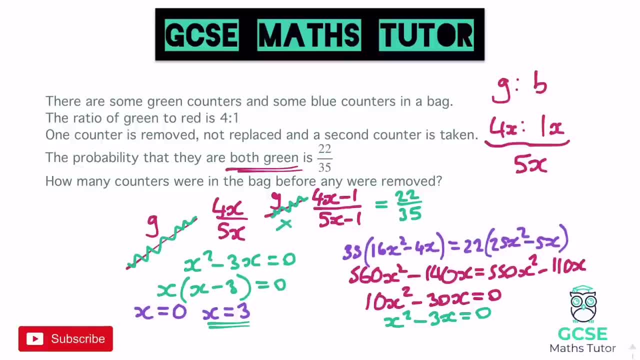 many counters were in the bag before any rule. Well, if we look back at this original statement here that we made, we said there were five x counters, or five lots of this x. So five times three, there we go would tell us that there were. 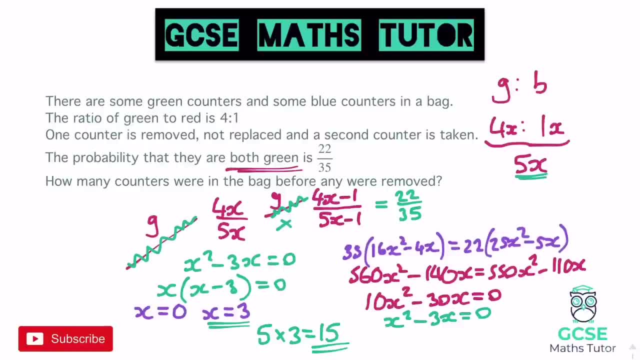 15 counters in the bag. Okay, it might have asked us how many green, in which case it'd be four times three, or 12 greens, and one times three for the blue, or three blues. Okay, so we've got 15. 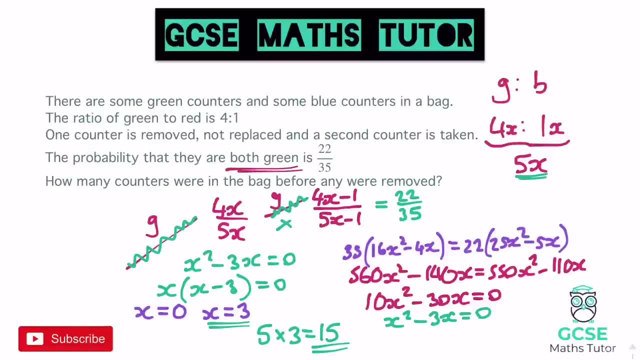 counters in the bag and that's the end of the question there. So you have to construct your two branches of the tree using expressions. So you've got some algebraic fractions Creating your two fractions either side of the equal sign. we've got to cross, multiply to make it a single line. equation Expanded it all out, made it equal. 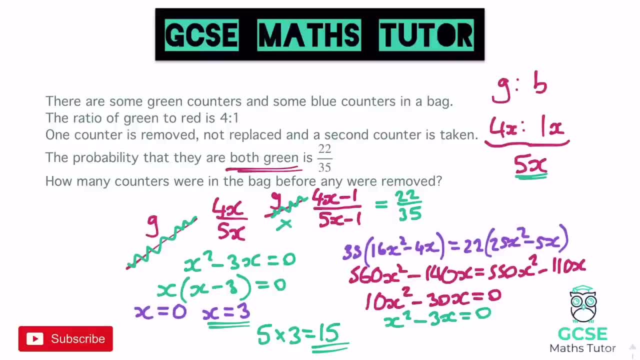 zero, solved it and then applied our solution to the question. So, as you can see a lot of maths going on there, But here's one that is very, very similar for you to have a go at see if you can get the answer for this one. Okay. so here's your question. Pause the video there. have a go. 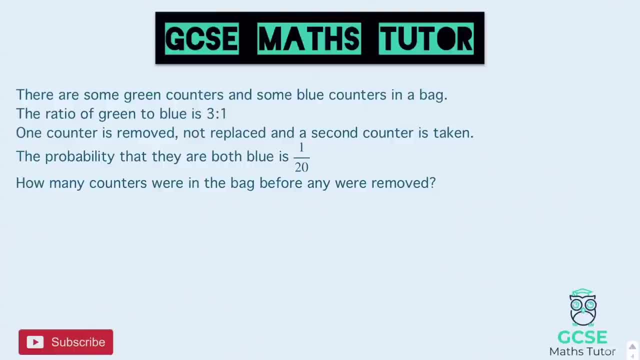 and we'll go over the answers in a sec. Okay, so we've got green to blue counters and it says green to blue is three to one. So if we label this up as a ratio, we have green to blue 3x, 2x and in total that gives us 4x. So constructing: 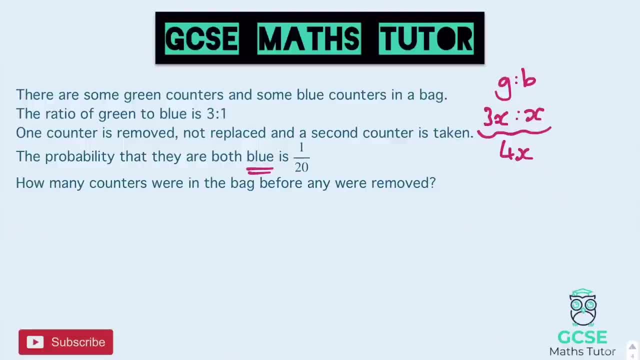 our tree. we're interested in the fact that they're both blue here. So if we have green going up, blue going down, keeping it in that same order, green would be 3x over 4x and blue would be 1x. 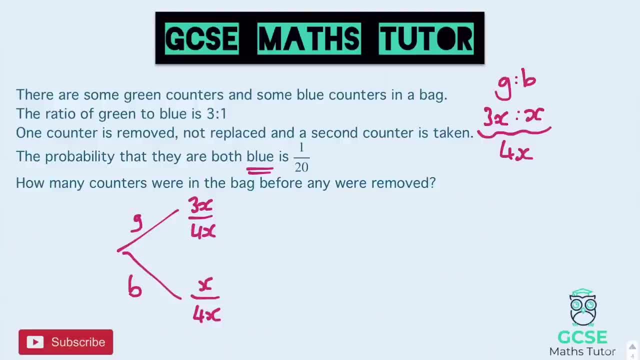 over 4x. Now I'm not going to construct the whole tree here, because what we're really interested in is blue again And blue. if we took one out, it would be x minus 1, and on the bottom there we would have 4x minus 1.. Okay, so I'm going to remove the top part of my tree there. 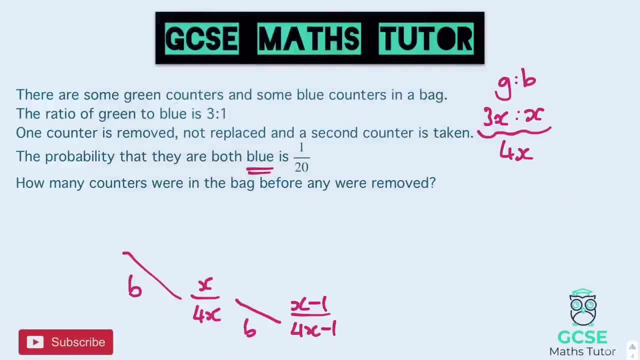 we don't need that anymore and we'll have a look at how we're going to construct this next part. So obviously, what we need to do is multiply these together, moving across the tree. So we have x over 4x and we are multiplying that by x minus 1. 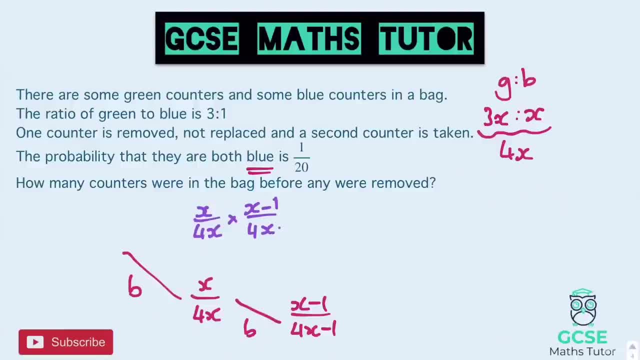 4x minus 1, and that's going to equal 1 over 20.. Let's go back actually multiplying these. So if we multiply those together, let's see what we get. x times x minus 1 on the top gives us x squared. 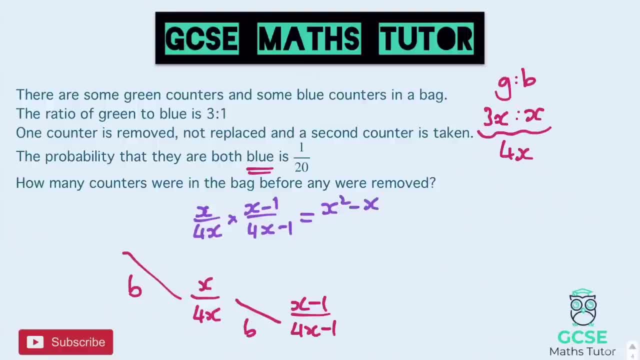 minus x and on the bottom, 4x times 4x is 16x squared and 4x times negative 1 is negative 4x. Now that fraction there equals 1 over 20.. And again, just like before, we just need to cross. 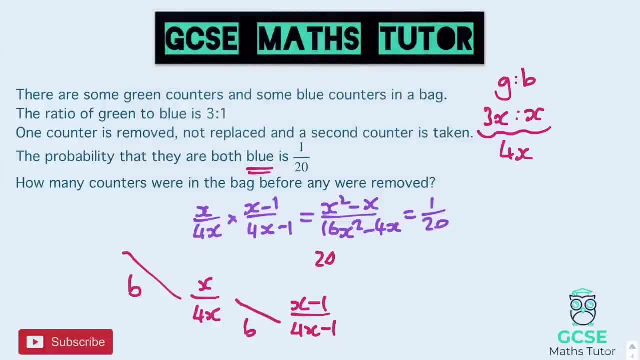 multiply, So times the left-hand side of the tree. we're going to multiply that by x minus 1,, top by 20, and we get 20, lots of x squared minus x and times the right top by 1.. So we don't. 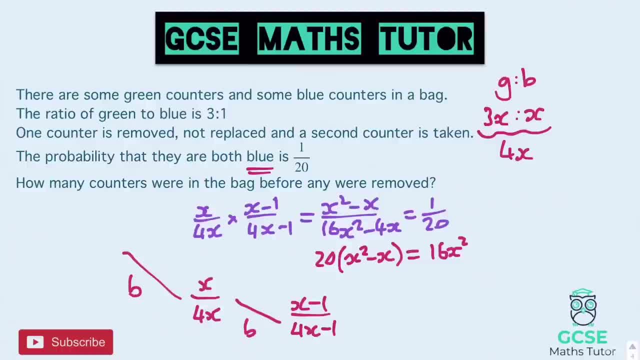 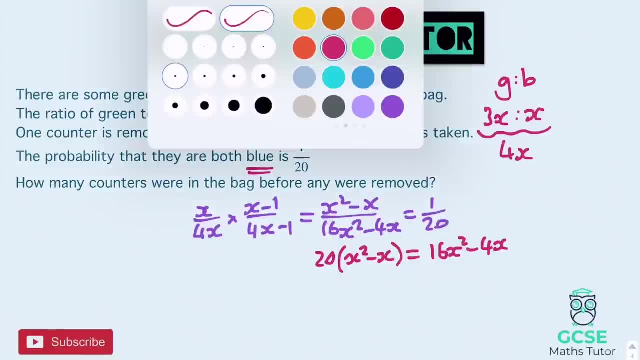 actually need to write that. it's just going to be 16x squared minus 4x. There we go. I'm going to get rid of this tree, so we have some room Right. so actually expanding this out if we go about. 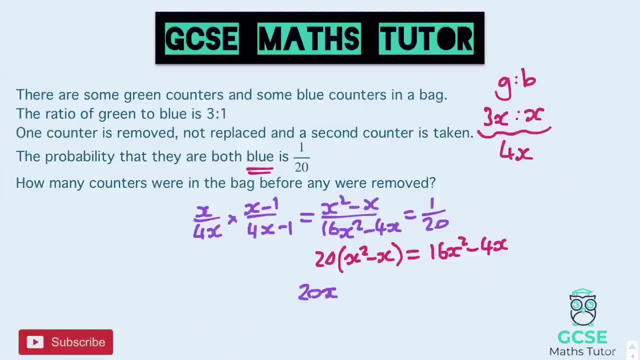 that we get 20x squared minus 20x, and that is going to equal 16x squared minus 4x. Now we need to make it equal to 0.. To set it equal to 0, let's minus 16x squared from. 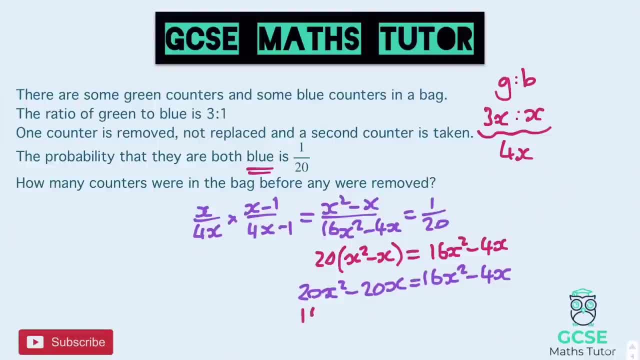 both sides and we get: oh, I've written 16 as well as taken it away. So 20x squared: take away 16x squared leaves us with 4x squared Negative 20. add 4 leaves us with negative 16, and now that? 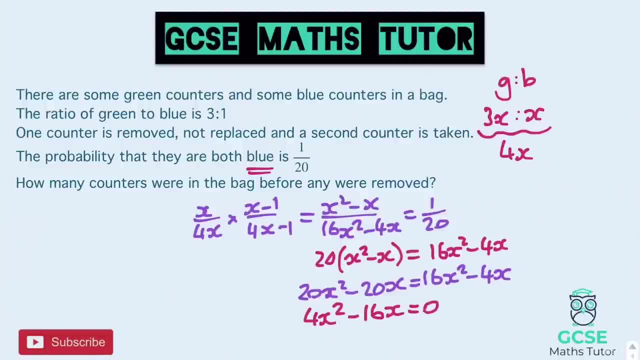 equals 0.. Again, we can divide both sides by 4 here. So if we simplify this down, divide both sides by 4, let's bring it over here- we would have 1x squared Minus 4x equals 0. Factorise it by x so we can solve it. So we get x minus 4, and then we get our. 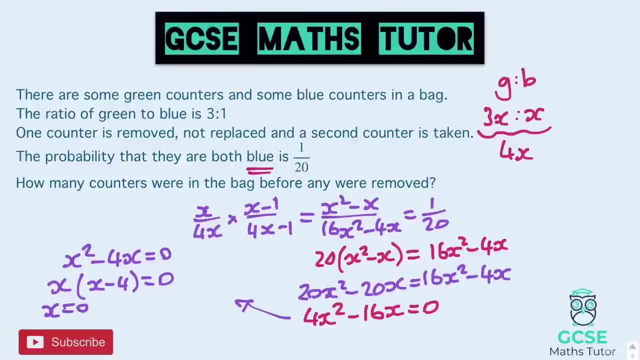 two solutions. So we have x equals 0 on the outside there and we have x equals 4 in the bracket. So there's our solution: x equals 4.. Again, it can't be 0. So how many counters were? 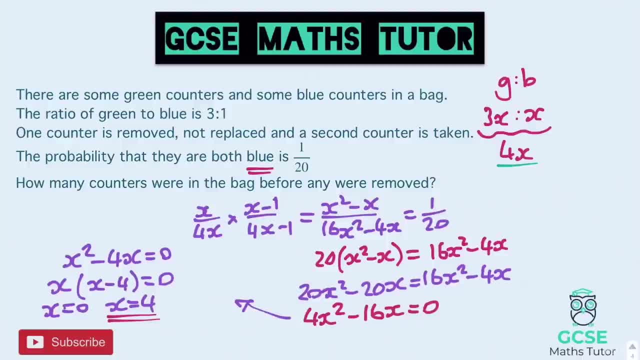 in the bag before Let's have a look. Well, we started with 4x up here, so 4 times 4, leaves us with 16 counters that are in the bag before we started. Again, 3 lots of x would give. 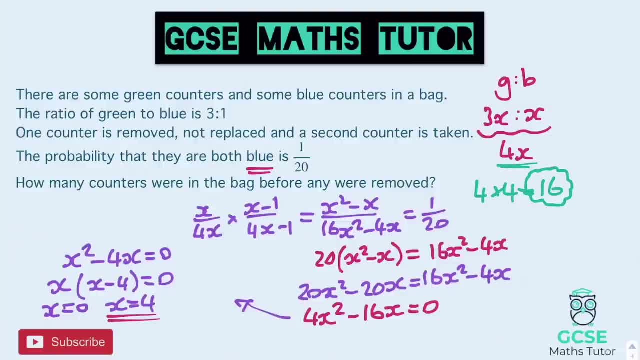 us 12,. 1 lot of x would give us 4, but the total amount of counters there is 4x. so 4, lots of 4 gives us 16.. Right well, now we're going to have a look at a slightly different question, Okay. 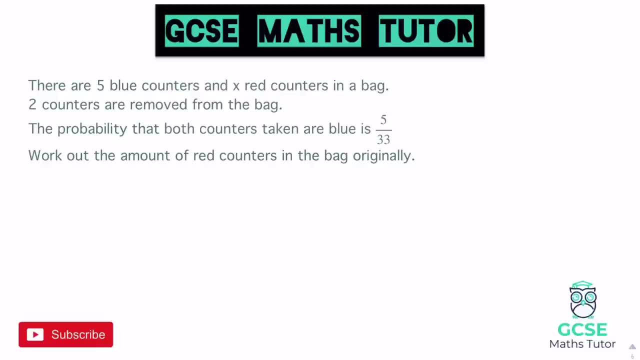 so we're going to treat this question exactly the same way, but we've got something slightly different going on here. It says there are 5 blue and x red. So again, if we write our ratio- this time blue to red- it is going to be 5.. 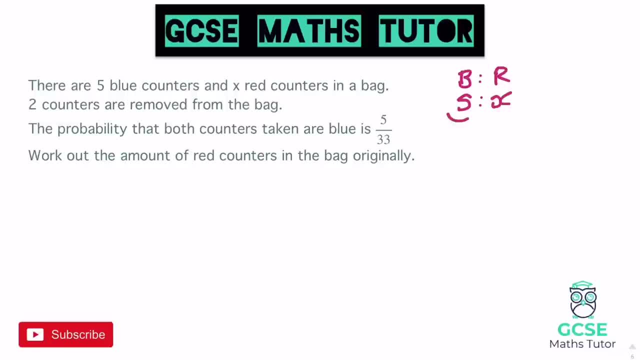 Blue to x. Okay, so our total this time is going to be 5 plus x, so I'm going to write it the other way. I'm going to write x plus 5.. I just prefer looking at it like that, although it doesn't. 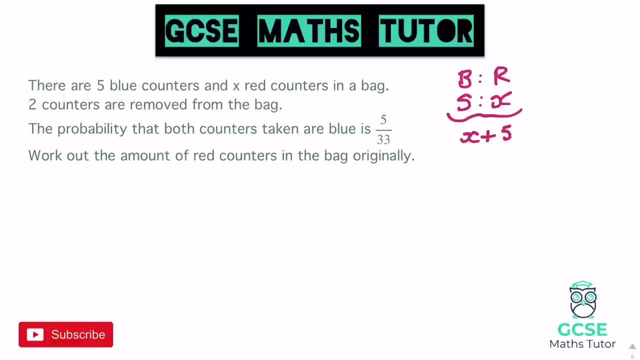 actually matter And that is going to be our denominator. Now it says the probability that they're both blue- okay, so that both counters taken are blue- is 5 over 33.. Work out the amount of red counters in the bag originally. So again, if we construct a tree here, we've got blue and 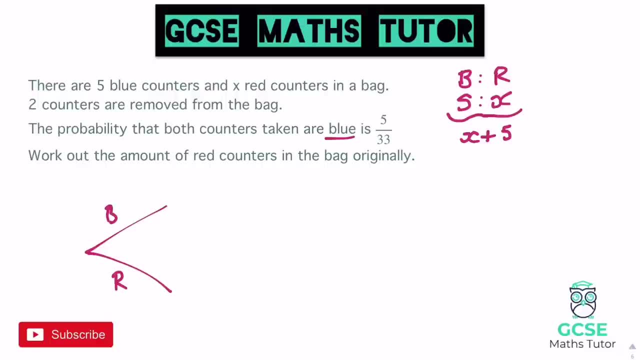 red, blue to red. I'm not even going to worry about filling in the red one this time and the. I'm just going to go for the blue. So blue. there are 5 counters and our total that we've worked out there is x plus 5.. Now one of the counters is not replaced, so the next time we take a blue. 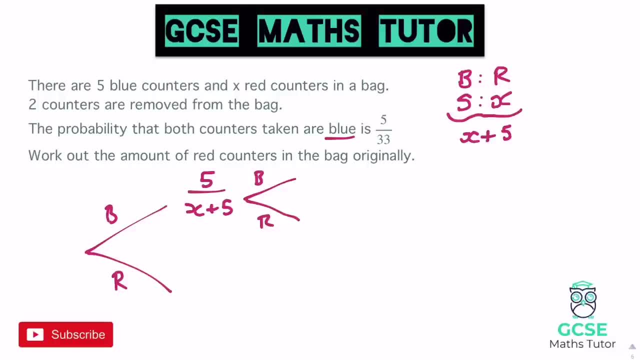 I'll think about drawing the tree here Again. I'm going to leave red out, But the next time we take a blue we'll take one away from the 5. there leaves us with 4 blues and take one away from. 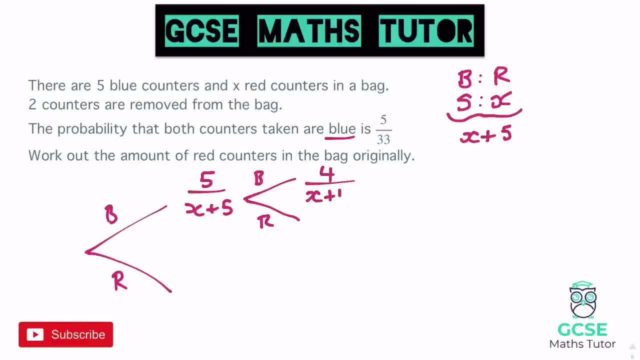 the x plus 5, leaves us with x plus 4.. So that is that part of the tree that we need. okay, We don't need the red roots here, so we can get rid of those. They're the only ones that we're actually. 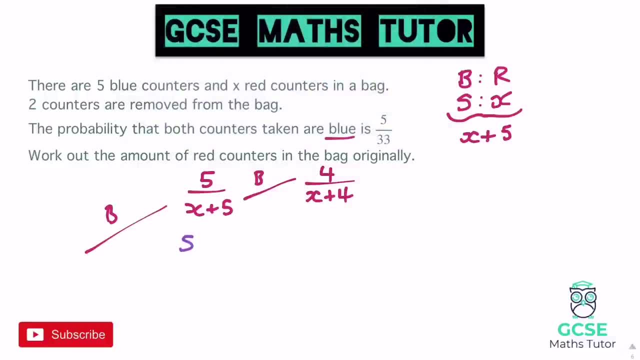 interested in. So if we have a look at timesing these together now, so we have 5 over x plus 5, and we're going to multiply that by 4 over x plus 4. And again that is going to be equal to 5 over 33,. okay, So 5 over. 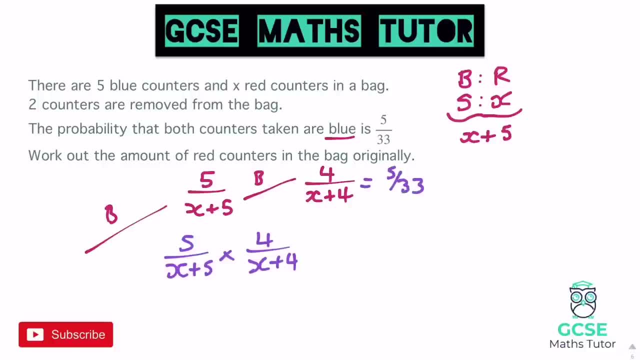 33.. But let's go about actually multiplying these first. So 5 times 4 on the top gives us 20, and then we've got a double bracket to expand on the bottom, So you can work that out to the side What. 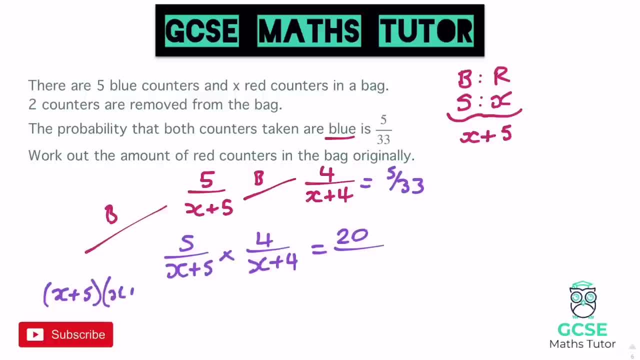 have? we got x plus 5 multiplied by x plus 4.. I'm going to expand this out quite quickly. We get x squared plus 9x plus 20.. And obviously, just take your time expanding that as a double bracket. 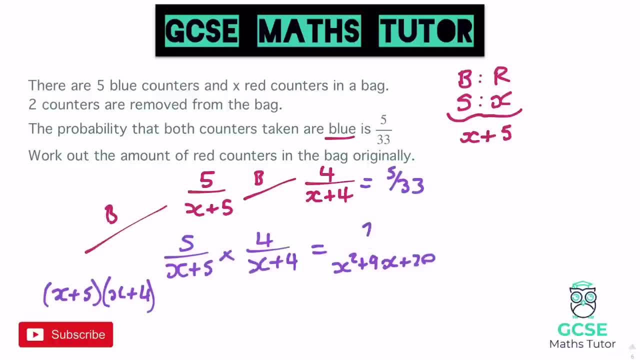 All right, let's tidy that up a bit, because that's a bit of a mess. Right, 20 on the top over that, And we've got that. that is equal to 5 over 33.. So we've got a very, very similar. 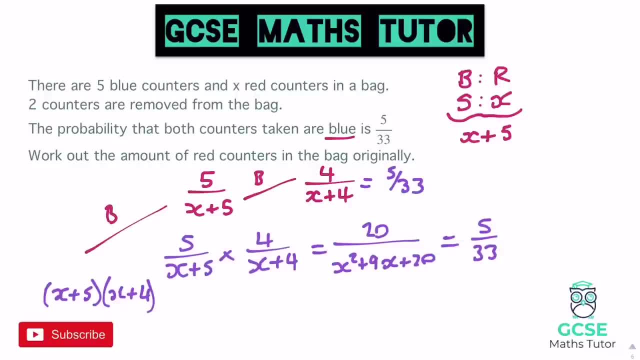 process here. Look, we're just going to times both sides by 33, and times both sides with this denominator here and cross multiply. So we're going to have 33 times 20 on the top, 33 times 20,. 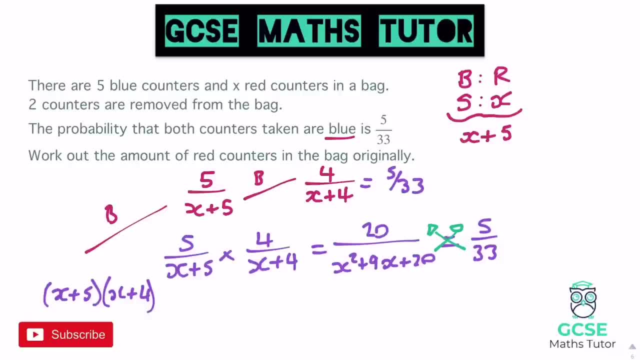 just doing this on the calculator gives us 660.. So we have: 660 equals 5x squared, plus 9x times 5,, which is 45x, and 20 times 5,, which is 100, so plus 100.. Okay, next step. 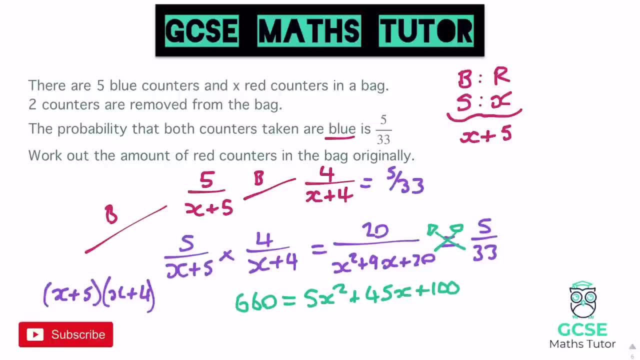 let's make it equal to 0.. So let's subtract 660 from both sides, So I'm going to write everything on the left-hand side. I'm just going to write 5x, 5x squared plus 45x Subtract 660 leaves us with negative 560, and that equals 0.. Now again, 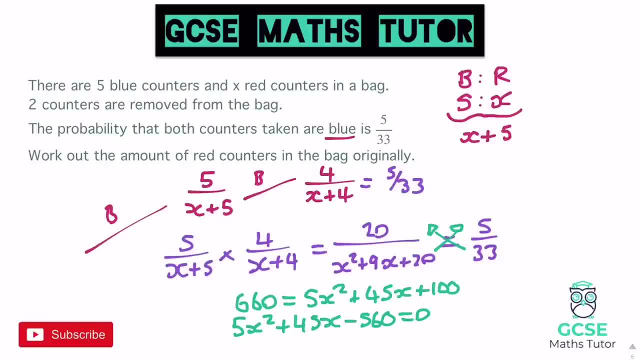 we've got a quadratic. I'm going to remove a lot of the working out here and let's just see where we're at at the moment. Okay, rid of all of that, Right? so we're at this point. So we've got a. 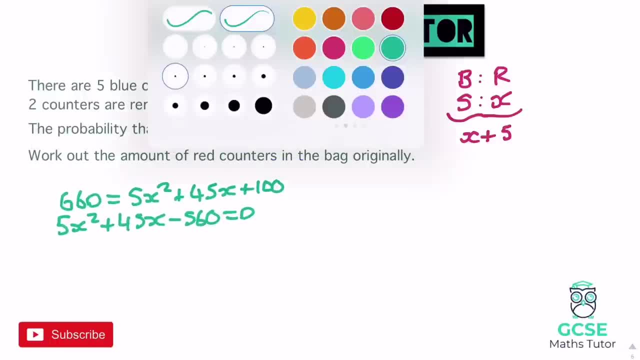 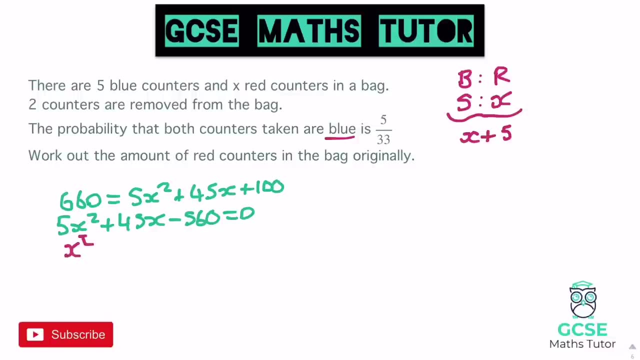 quadratic. We just need to make this a little bit more simple So we can divide everything by 5.. So if I divide everything by 5, because they're all multiples of 5, we get x squared plus, 9x minus, and 560 divided by 5 is 112, minus 112 equals 0.. Now again, I've shown you quite a. 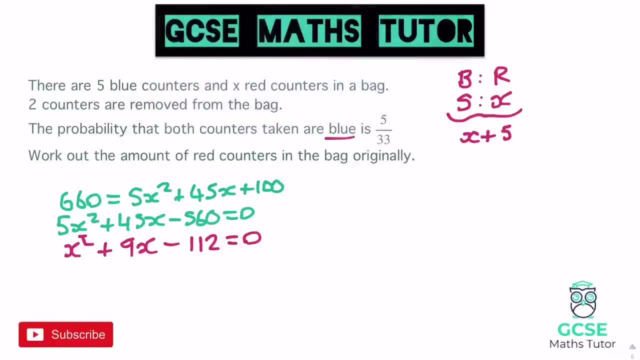 tricky one here because that's obviously not the nicest to factorise there. but if we factorise this it's going to go into a double bracket. Obviously, if you've got a calculator, this is quite nice because you can use the quadratic formula. but I'm going to assume we don't have 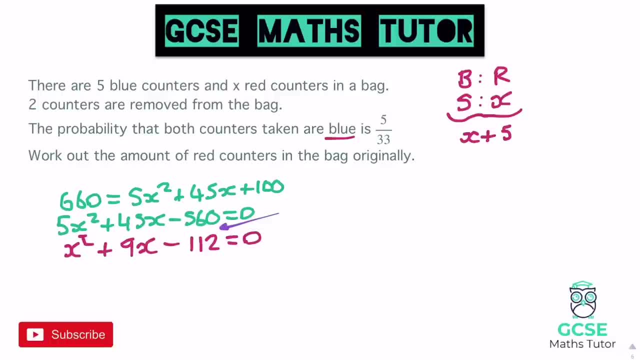 a calculator at this point. We're going to try and do it again. So we're going to do it again and we're going to factorise this. So the factors of 112, we can have 1 and 112.. We could have 2 and. 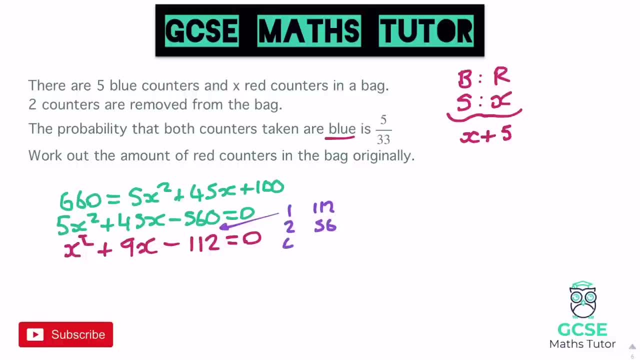 56. Let's have a think We could have 4 and 28,, or we could have 8 and 14.. Are any of these going to make 9? It doesn't look like it so far. What else goes into 112? Let's have a think We could. 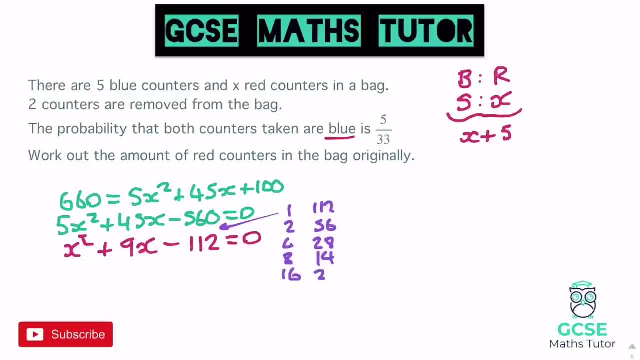 have 16 and 20.. Oh no, 16 and 7,, isn't it Okay? 16 and 7.. There we go Again. I am just using a double and half method here to find all these factors. So 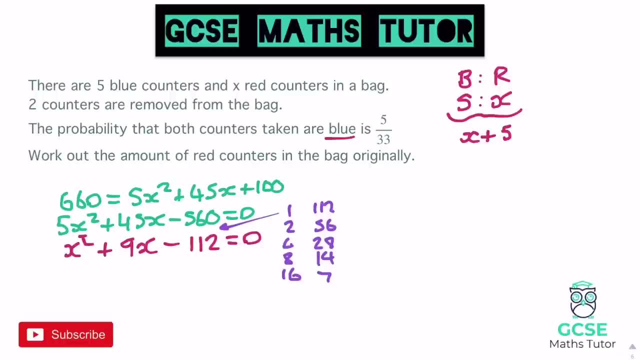 I'm doubling 8 and halving 14 to get my next factors there. So 16 and 7 can make 9.. So to make 9 in the middle, that would have to be x plus 16 and x minus 7.. Okay, and that all equals 0.. 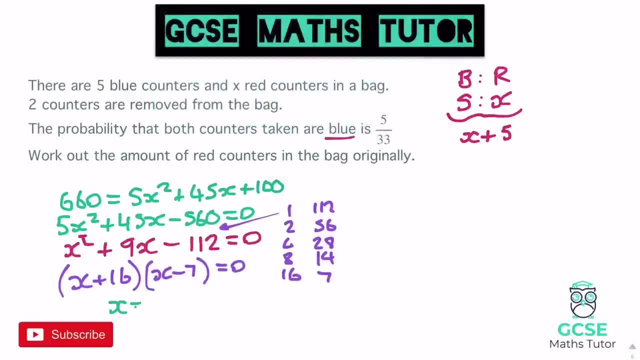 So we've got two solutions going on in the brackets. here We've got x can either be negative 16, or x can be positive 7.. Okay, obviously, again thinking about this logically, we can't have negative 16 counters for the reds. 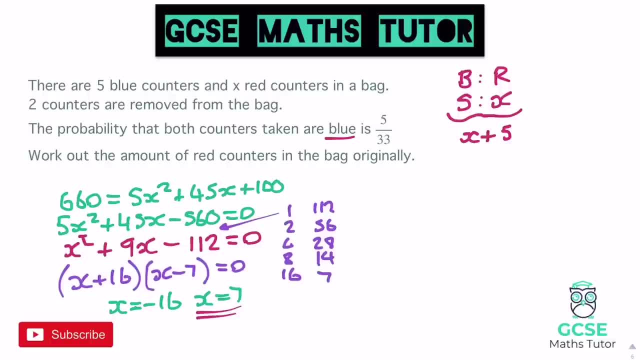 So there must be 7 reds in there. x was red, so x equals 7.. And we would just write red equals 7. And that would be our final answer. there Again, it could have asked us how many counters in total were in the bag. originally That'd be 7 plus 5. That'd be 12. But it's just asked us for. 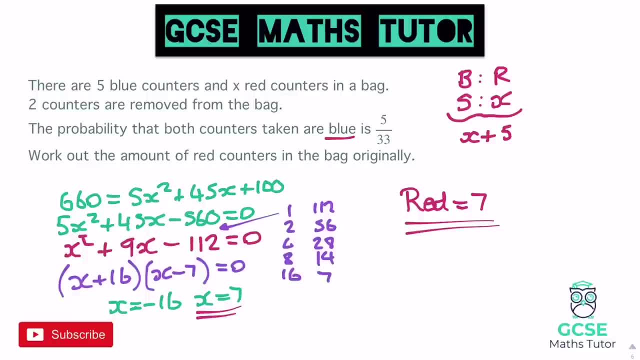 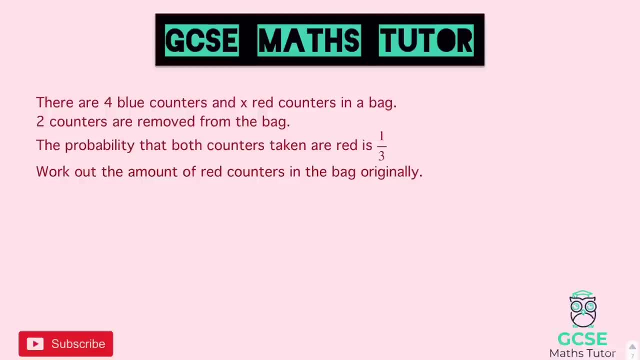 how many red? Okay, so there we go. There's our answer for that one. Okay, now you're going to have a go at one very similar Nicer numbers, but here it is. So here's your question. Pause the video there. We'll go over the answers in a sec. Okay, so there are four blue counters. 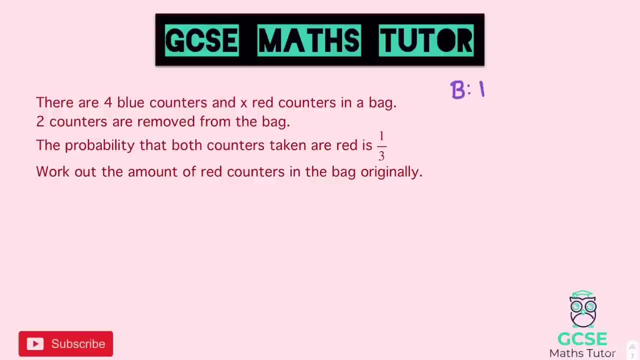 and x red counters. So if we write this as a ratio again, blue to red, we have 4 to x And in total there that is x plus 4.. Now if we write this as a probability tree, it says the probability. 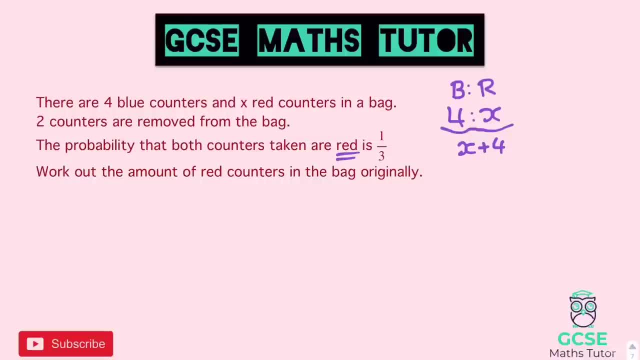 that both counters are red is a third. So I'm only really interested in the red root. I just have red going up just to save a bit of space here. It doesn't really matter which way we draw it, But red is going to be x over x plus 4.. 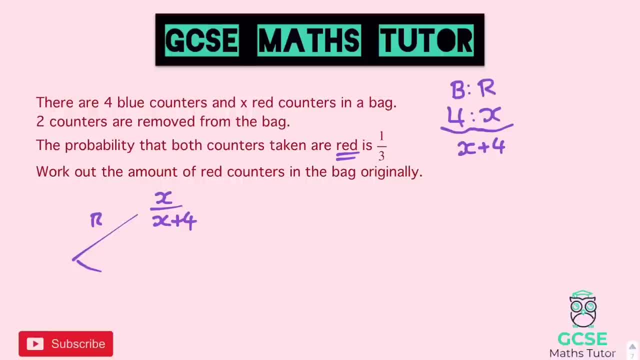 Okay, we don't need to worry about blue, And then red again would be x minus 1, because we're taking one red counter out And that'd be x plus 3 on the bottom, because one of those counters is gone. So it's not x plus 4 anymore, It's x plus 3. And if we times these both together, they're. 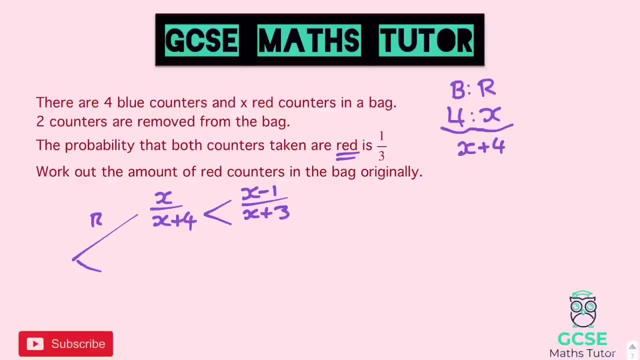 going to equal one third of that fraction given to us there. So x times- and you can always put a little time sign here- x times x minus 1 gives us x squared minus x And on the bottom we have a double bracket again. And if we expand that double bracket we have a double bracket again. 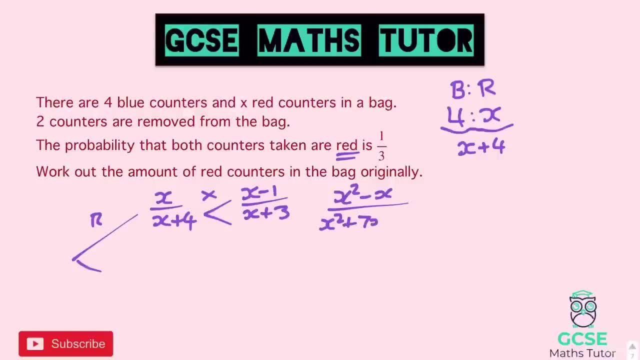 We get x squared plus 3x plus 4x, which is 7x plus 12. And that equals one third, And again cross multiplying. So times this top by 3, and this over here to the 1. And we get 3, lots of x. 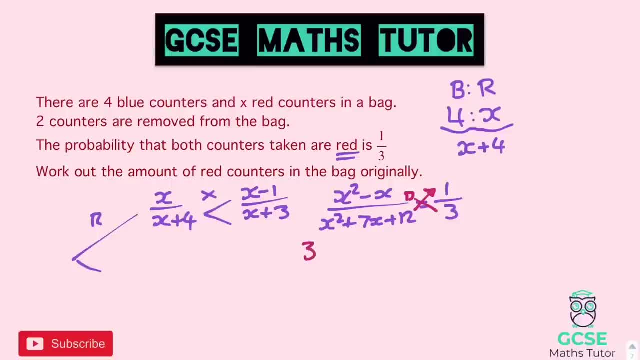 squared minus 3.. And you can always just imagine that I'm going to skip the step of writing it as a bracket. We've got 3x squared minus 3x, And that equals 1 times that denominator there, which is: 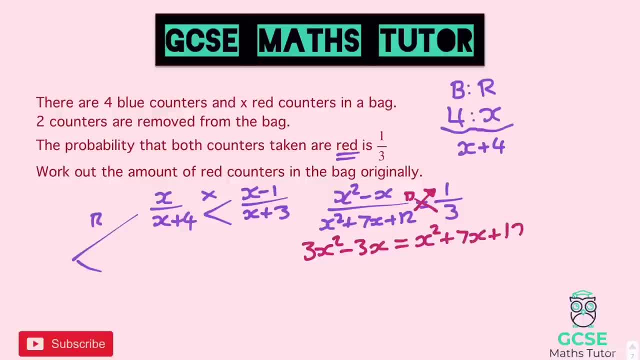 x squared plus 7x plus 12.. And then again just making this equal 0. So that's minus x squared from both sides to get rid of this one And that gives us 2x squared. That's minus 7x from both. 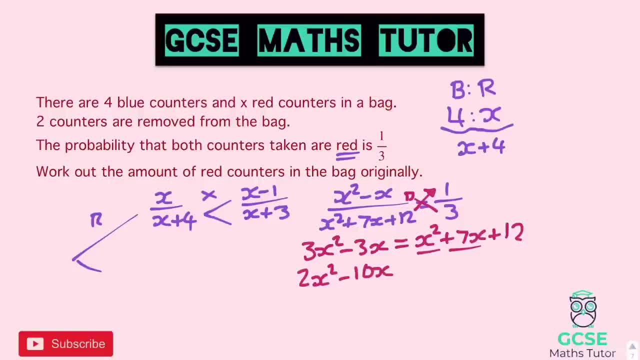 sides, which leaves us with minus 10x, And that's minus 12 from both sides, which just leaves us with minus 12, because there's no numbers over there, And now that equals 0.. Now again, they're all even, So we can divide them all by 2.. So we can have x squared minus 5x, minus 6, which equals. 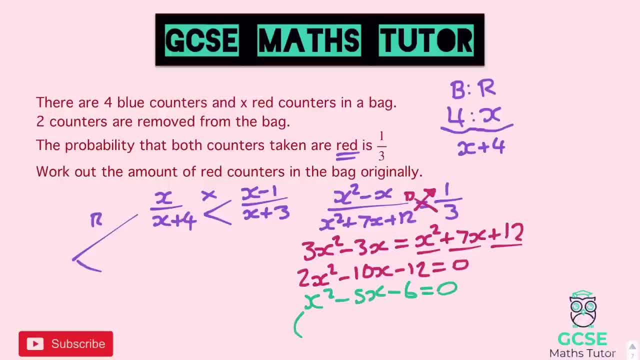 0. And that's quite a nice one to factorise there 3 and 2 times to make 6. And they can subtract to make negative 5.. Or we could have 6 and 1. Again, so always just make sure you write. 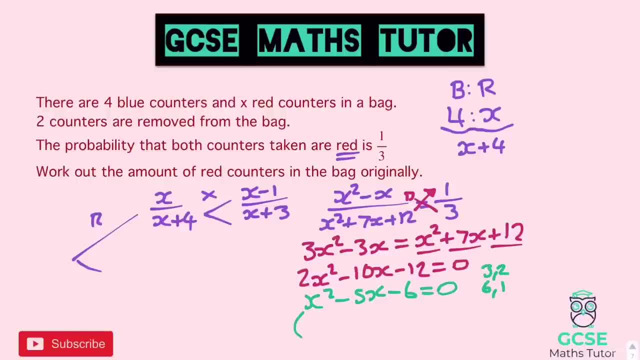 down the factors. We can have 3 and 2, or 6 and 1. And the combination that's going to make negative 5 there, which also gives us negative 6.. We're going to need x minus 6 and x plus 1. And that 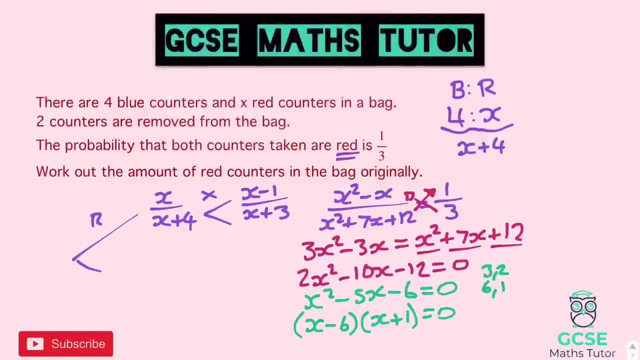 all equals 0.. There we go. So we've got two solutions there. We've got x equals 6, or x equals negative 1. And in the case of the context here we can't have negative 1 counters, So x is going to have to equal 6.. It says: work out the amount of red. 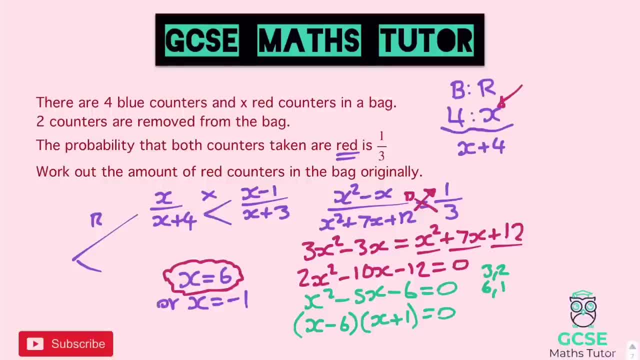 counters. Well, the red was just the x there, So x equals 6.. And 6 is our final answer. Again, we already knew that there were four blue counters, So now we know there are six red and that is 10 in total. So that's solving that one Again. if you weren't sure on any of 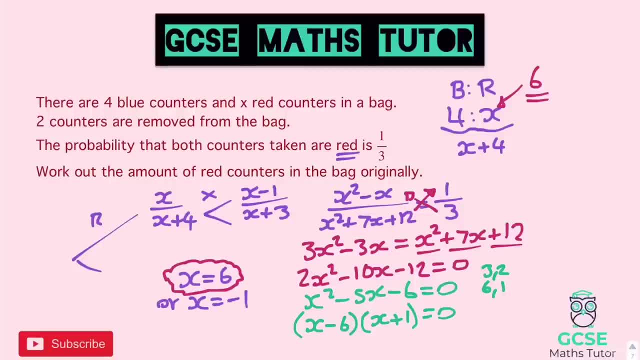 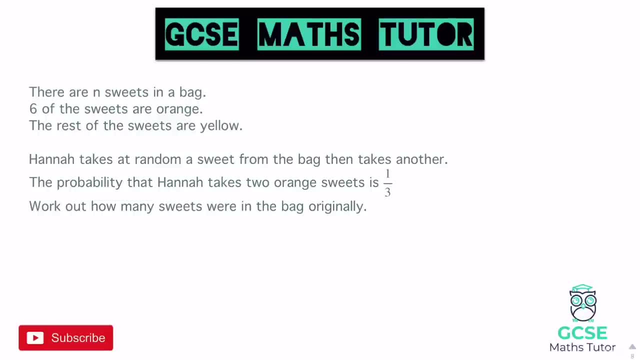 these. just go back, have another go. Make sure you've made some good notes on it. I've got one more question for you to have a look at before we finish. Okay, so you might have heard of this question or a similar question like this. It was quite a popular question. It was one that people 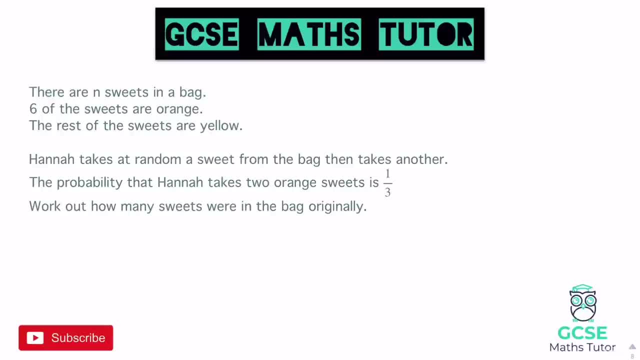 really struggled on. So it says that there are n sweets in a bag. Six of the sweets are orange and the rest of the sweets are yellow. Hannah takes at random a sweet from the bag and then takes another, And the probability that Hannah takes two orange sweets is one third Work out. 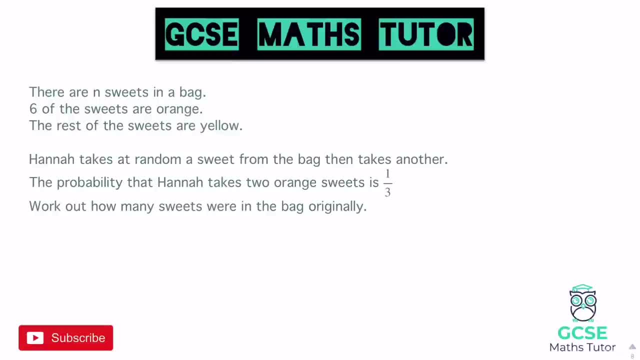 how many sweets were in the bag originally? So n sweets in a bag. six are orange, rest are yellow. She takes a sweet at random, doesn't replace it, takes another. and then the probability that two orange sweets is one third. This is different to the other two that 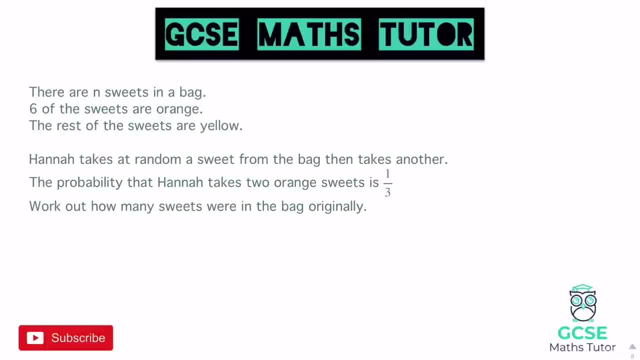 we've done, but it's all a very similar process. It's solved in exactly the same way. So have a go see if you can figure this one out, And we're going to go over the answer, but just see if you can create one after me not going over one that's super similar to it. So you've got enough. 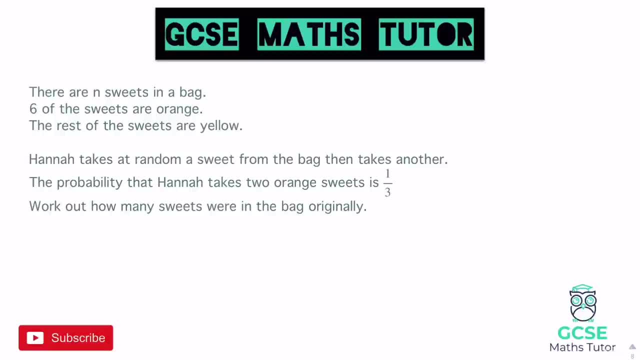 information there off the previous ones that you've had a go at, to have a go at it. So have a go see what you get, and we'll go over the answer in a sec. So pause the video there. Okay, the answers for these then. So there are n sweets in a bag, So this time it's given us our. 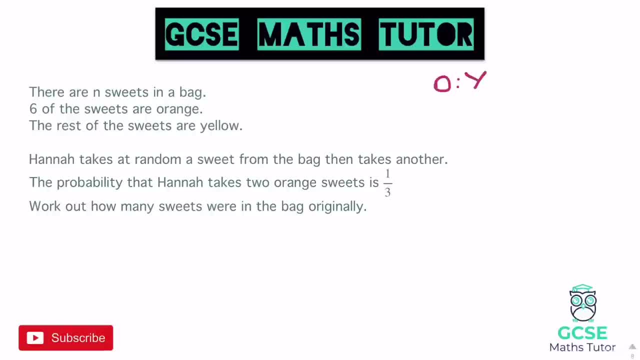 total And the option is either orange or yellow And it says that there are six orange but it doesn't tell us how many yellow, It just says that the rest of them are yellow. Now we know the total is n because it says n sweets in a bag. So the total, take away the six for the orange would leave. 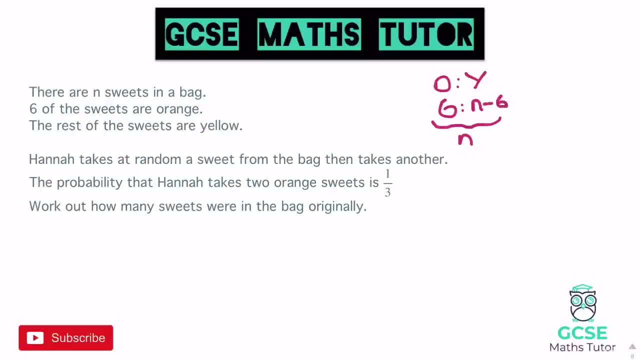 us with n minus six for the yellow. So a little bit different here, because yellow is n minus six, the total take away six. Now we're only interested in the two orange sweets And if we think about constructing our tree, and again we only need the orange root, orange would be six over n And 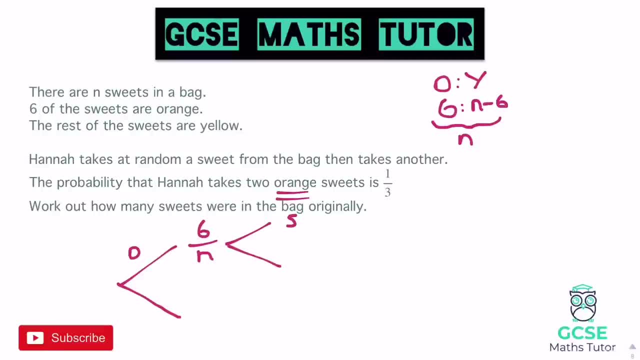 then another orange would be five, six. take away one over n minus one. So, as it turns out, we don't even need to use that n minus six. But it's always good just to think about what the expressions would be either way, because we could be given the probability of two yellows, but actually this one. 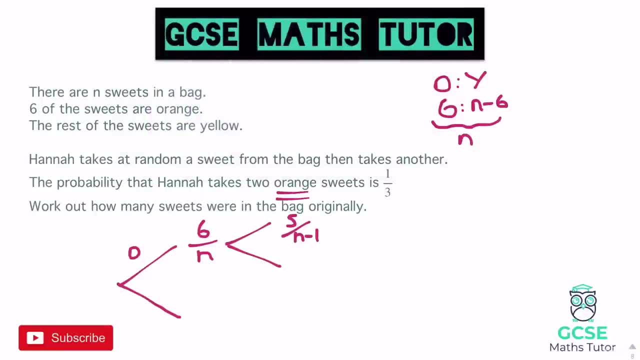 wasn't too bad. So if we go back, actually times in these together, they'll equal a third. So six times n minus one, which is n squared minus n, And that equals one third. Again we're at the point where we can cross multiply. So we'll times this up here and we'll times the three up there And we: 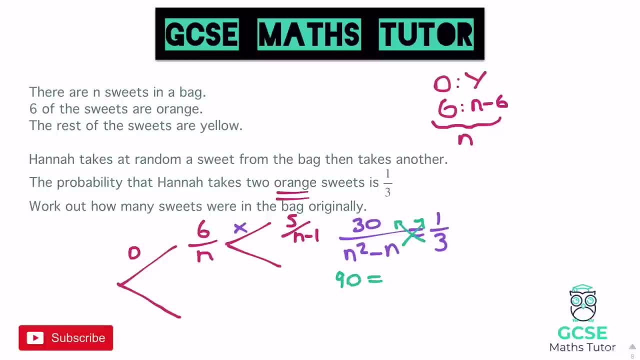 get 90, three times the 30 equals. so it's only one times the denominator here. So it's n squared minus n. Let's make it equal zero. I'm going to go minus 90 from both sides, So zero equals n squared. 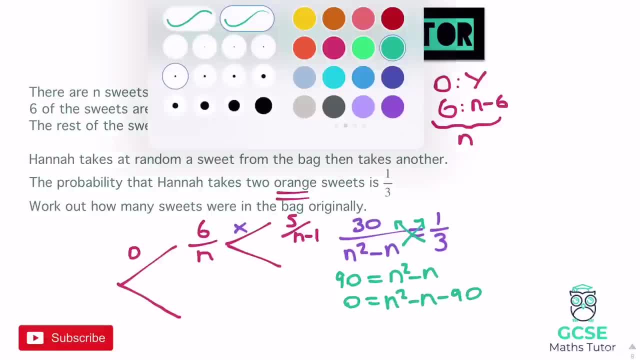 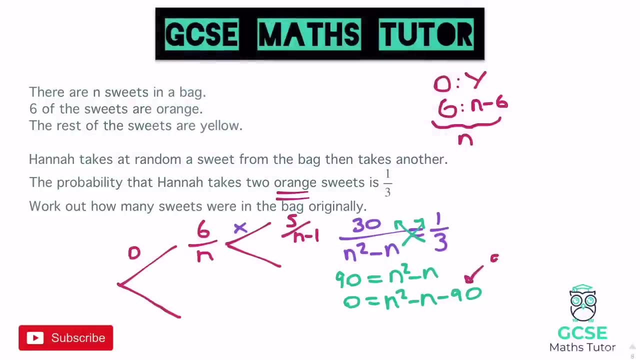 n minus 90. Again, you can write that the other way around if you want, but I'm just going to factorise it from there. So the factors that make 90, we could have lots, but we're trying to make negative one in the middle And that option there is going to be nine times 10. We're trying to make 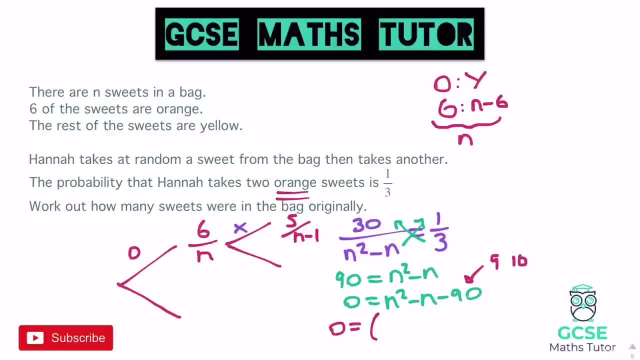 negative one. So we'll have naught equals, it'll be n to make negative one. we want plus nine minus 10.. So n minus 10.. And again, we've got our two solutions there. So we've got the option is: 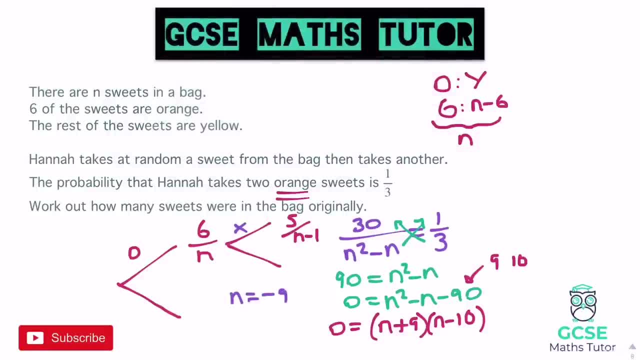 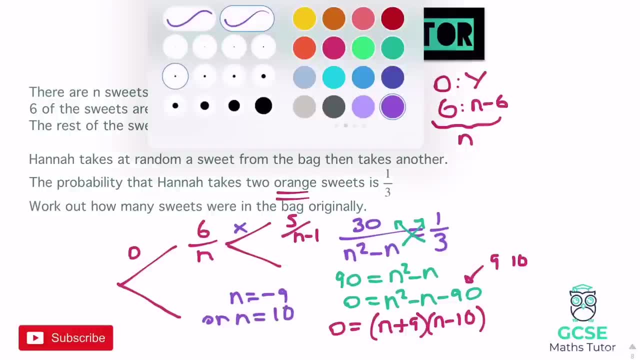 n equals negative nine Or n equals positive 10.. Okay, obviously, thinking about the context here, it's got to be the positive one, can't be the negative nine. So n has to equal 10.. Now it says: work out how many sweets were in.